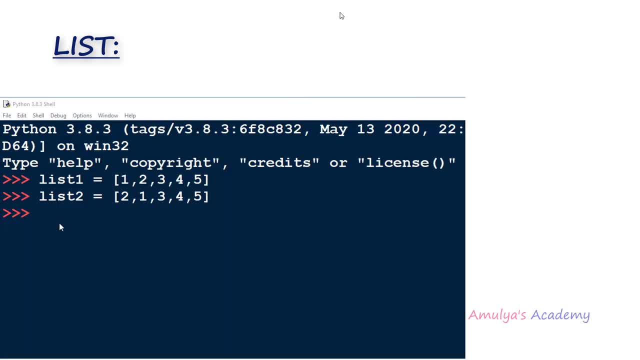 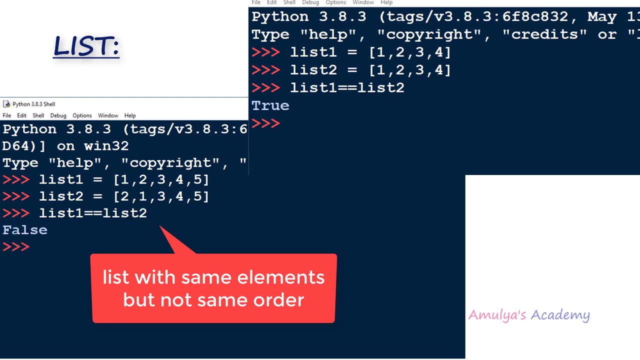 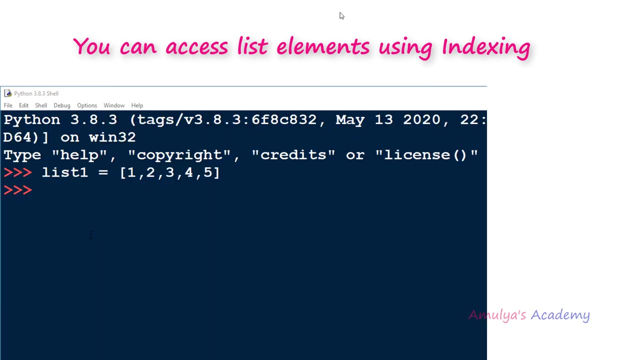 after the removed element change their index position, but the order will remain same If the list has different order. here we can see they are not equal. List elements can be accessed by index. list indexing is zero based indexing. that means the first index of the list will be zero, next will be one like that, the starting index. 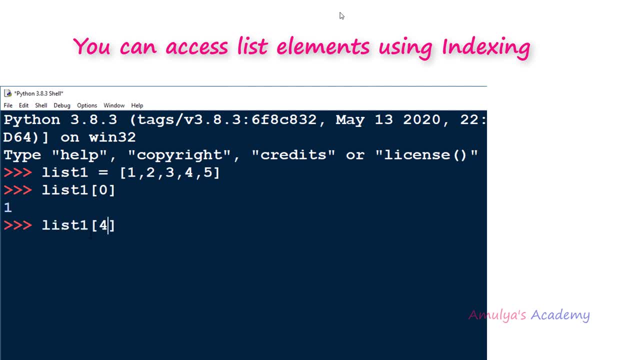 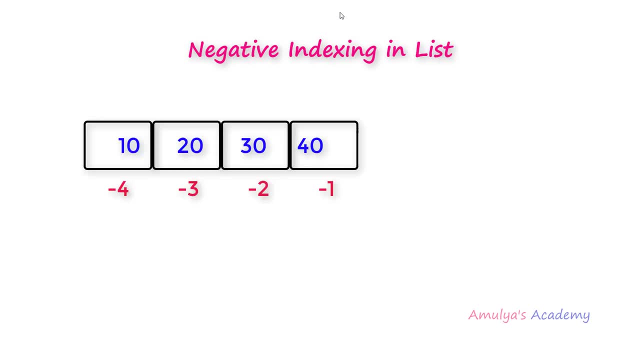 of list is zero, so that's why it's called as zero based indexing, and if you want to access any element from the list, you can use the index of that element. You can use negative indexing also. like positive indexing, you can use the negative indexing. 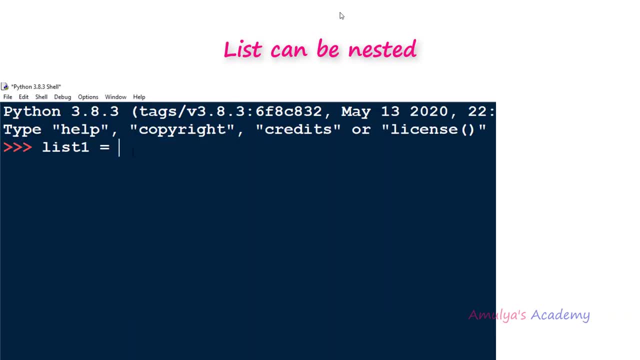 also, List can be nested so you can have list as the list element. you can have list inside the list. as i said, in the list we can have the data of different data type. we can have list also as the element of the another list. 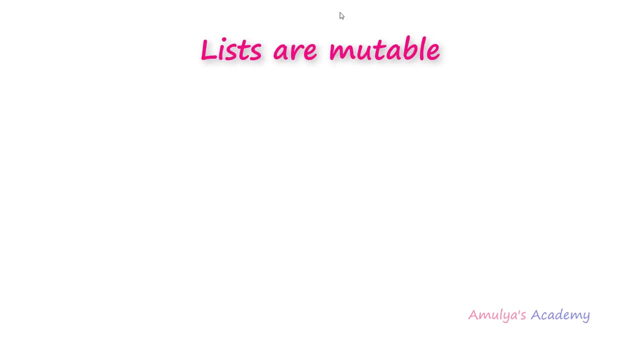 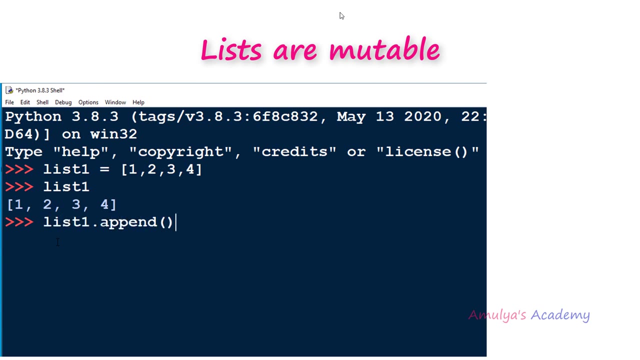 So list can be nested. list are mutable. after creating a list you can modify that. you can insert any element or you can delete any element from the list. you can modify that. that's why list are called as mutable. So there are different list method. we already discussed about that. i will give you the 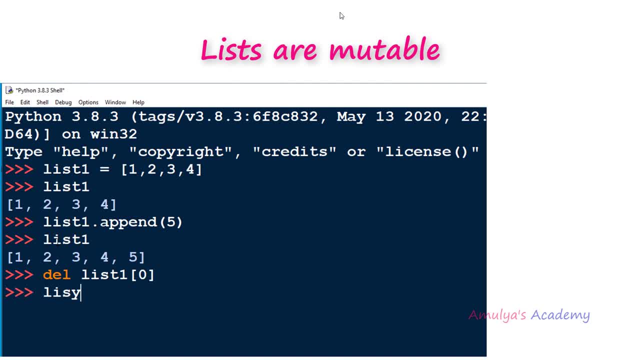 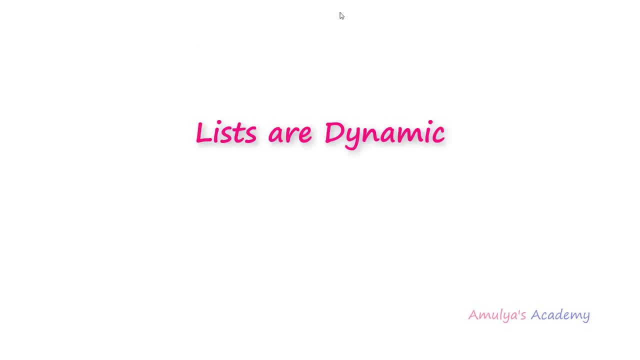 link of that video in the description box. you can go and check that. using that, you can insert, append or delete the element to the list. Next, lists are mutable. List are mutable. Lists are dynamic. When we add element to the list it will grow. when we delete the element, it will shrinks. 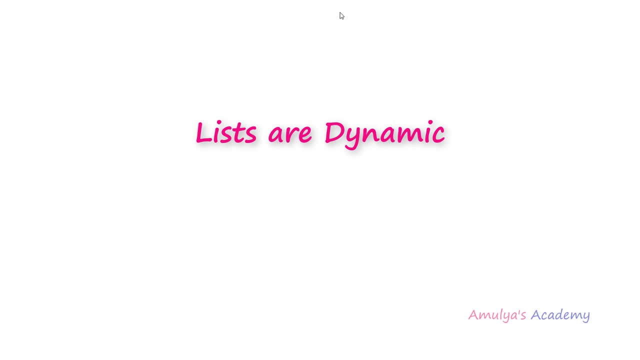 right, because list is mutable. we can add the element or we can delete the element after creating that, Ok. so this is about the list, because we already discussed about this concept in detail. that's why i am not explaining more about this. i will give you the link of previous videos. 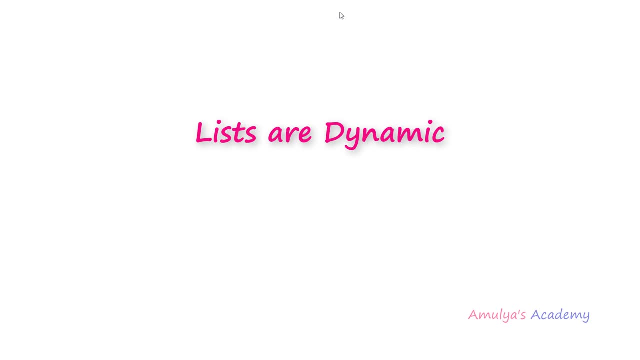 in the description box. you can go and check that if you want detailed explanation. Next let's talk about the tuple. Tuples are also stores, the collection of different type of data. it is similar to the list, but it has few difference. Tuples are comma separated elements enclosed within the parenthesis in the list. elements. 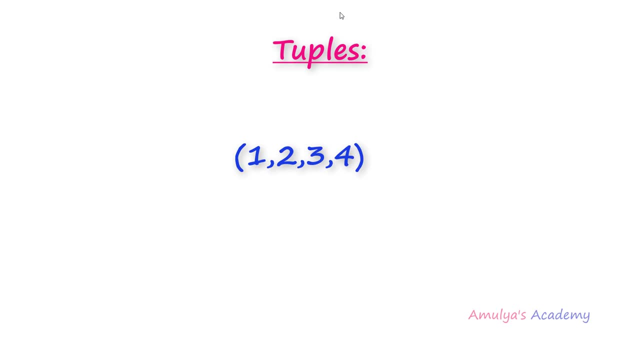 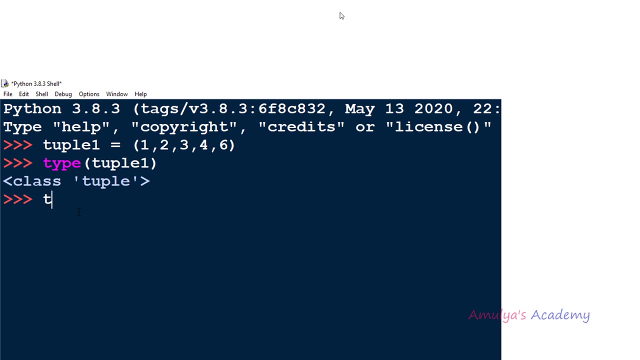 are enclosed within the square brackets, but here in the tuple, the elements are enclosed within the parenthesis. if you didn't use parenthesis also, the value separated by the comma are called as tuple. Ok, So here we can see the example and you can create the tuple using like this: you can. 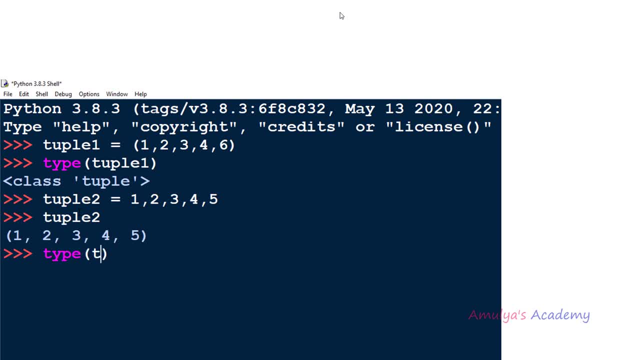 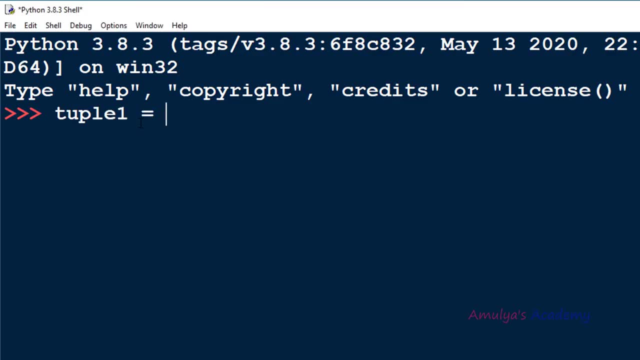 take a variable and you can take the parenthesis inside that, you can take the elements or you can use the tuple constructor also you can create the empty tuple like this, but because we use parenthesis for grouping also in python programming language, so we may face few ambiguities. 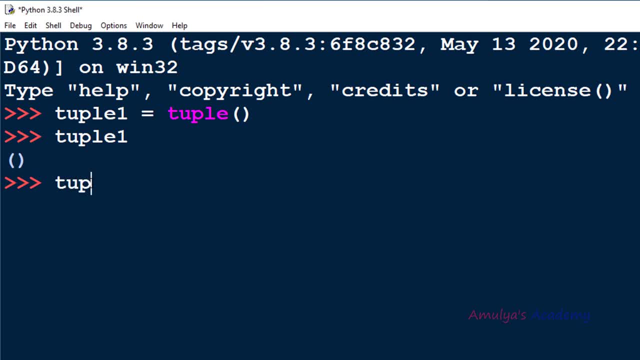 the confusions. that is when i take a single element in the tuple. if you initialize like this, here we can see the type of the tuple. it is not tuple, it is a integer value, because i enclosed within the parenthesis it will not treat that as the tuple, but it will treat. 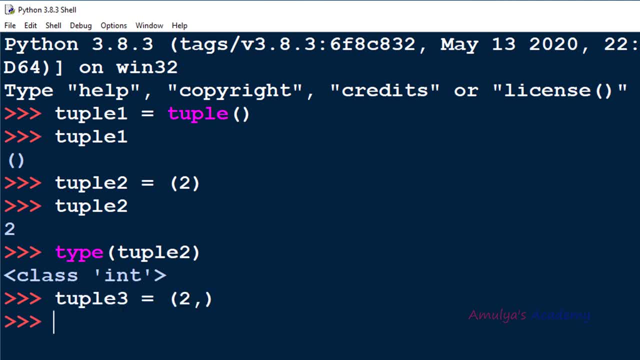 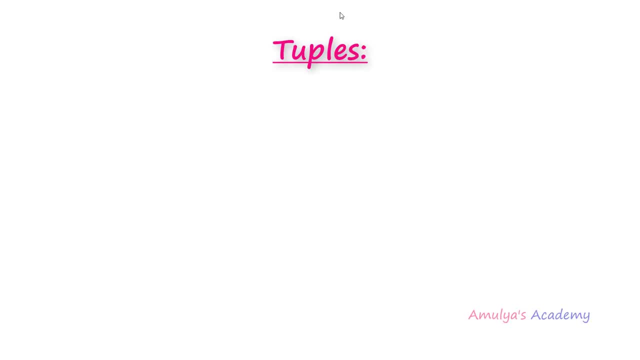 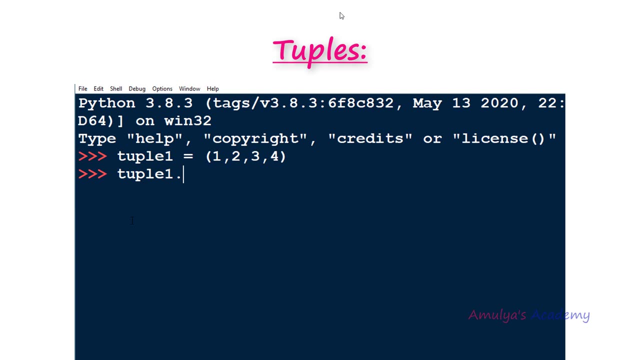 that as a grouping operator. So to create a tuple with the single element, include a comma here after the value. Next difference is Tuples are immutable. list is mutable. right, it can be changed. after creating the list we can modify it. but after creating the tuple we can't modify it. we can't insert the. 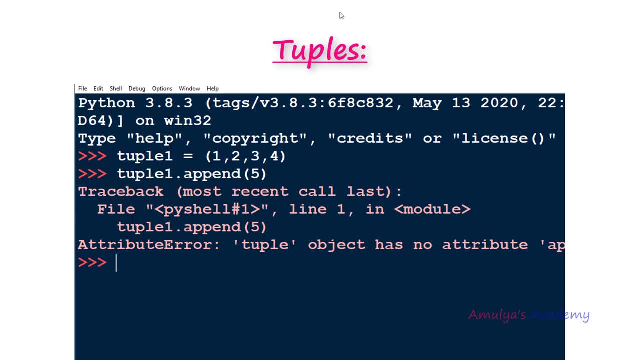 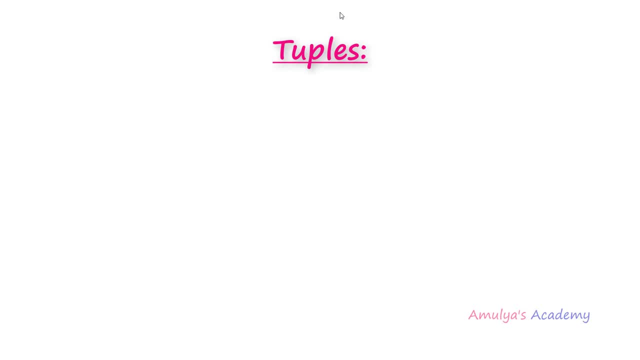 element, or we can't delete the elements from the tuple, so tuples are mutable. So next see the similarities between the list and tuple. which characters are similar between the list and tuple? Tuple also stores the collection of zero or more number of element, and here the elements. 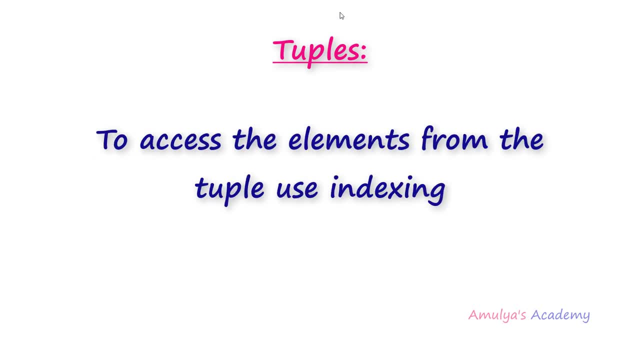 are separate. To access the element from the tuple we need to use the index here. tuple indexing also zero based, that is nothing, but the first element index will be zero. here also you can use the negative indexing. tuple can also be nested so you can use the tuple inside. 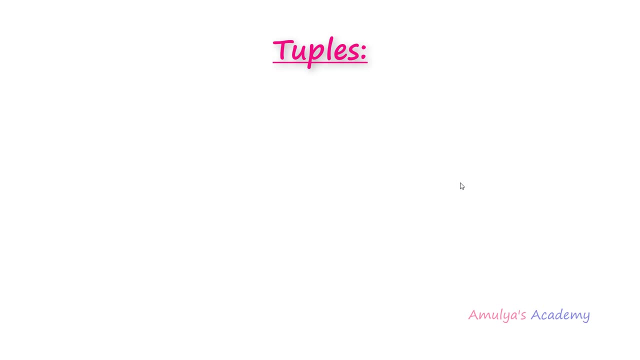 the tuple. So next, why we need tuple when we have list. That is because tuple is faster than the list and also sometimes you don't want data to be modified If the values in the collection are meant to be remain constant for the life of the. 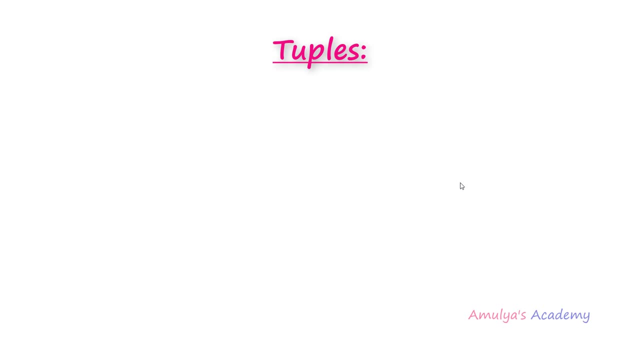 program. using a tuple instead of list guards against accidental modification. Ok, so this is about the list and tuple. if you want detailed explanation, the video link is in the description box. In the next tutorial we will discuss about set and dictionary. So that's it for now, guys. thank you for watching. don't forget to subscribe to my channel. i will meet you in next class. till then, take care. 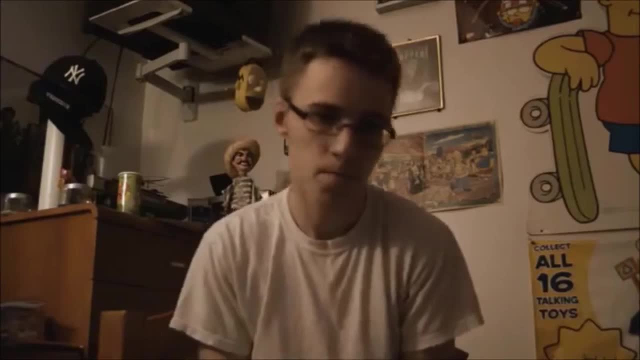 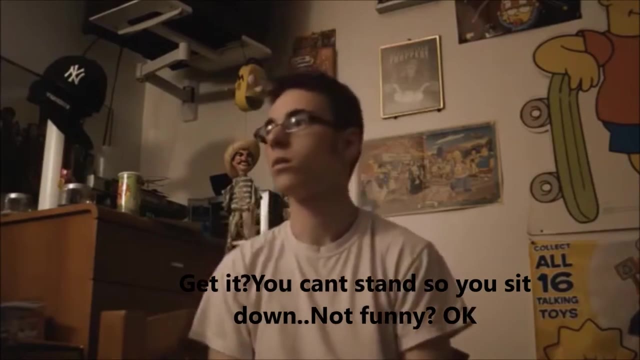 If you ever have a class that you just can't stand, so you sit down, instead you get it. you can't stand it, so you sit down. What was it, honey? Ah, okay, Two plus two is four. we ain't doing it anymore. I got 99 thumbs, but Calc ain't one. it's about 90 of them, son. 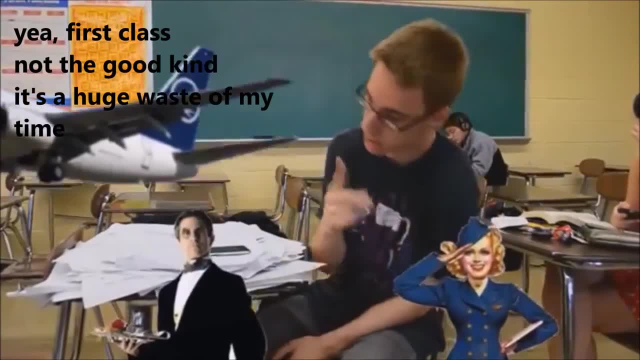 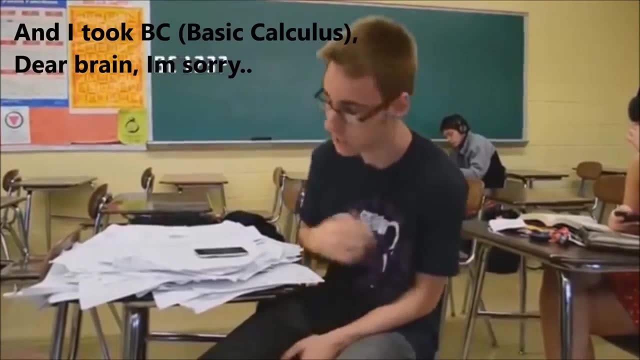 That's how I start my day. I wake up at 7 am. yeah, first class and not the good kind. it's just a huge waste of my time. Decided to take AP. what the hell is wrong with me? and I took BC. dear brain, I'm sorry. 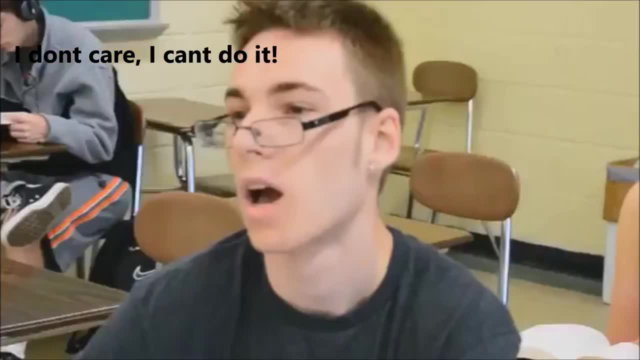 Man, I wanna quit, wonder when I'll ever need this. I don't care, I can't do it. This is so queer, everything is unclear. I'm not an agent sittin' here hopin' for an alien invasion. 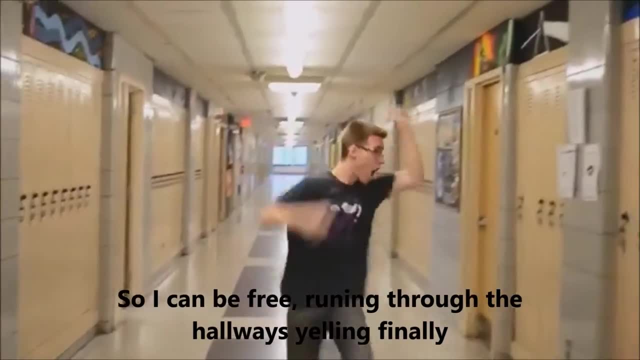 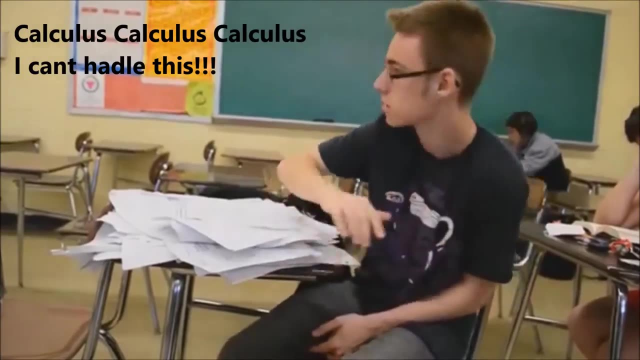 Take over the nation so I can be free. we're runnin' through the halls yellin' FUNNY ME. Calculus, calculus, calculus. I can't handle this. Calculus, calculus, calculus. I can't handle this.